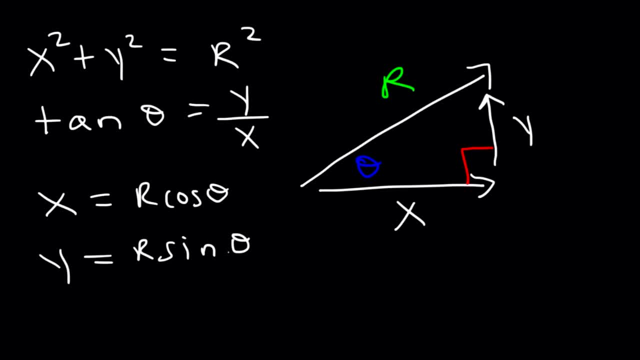 on some examples so you can master your ability to convert a rectangular equation into a polar one. So let's start with this example. Let's say that x is equal to 8, and that's because we're going to go ahead and take a minute, convert this rectangular equation into a polar equation. 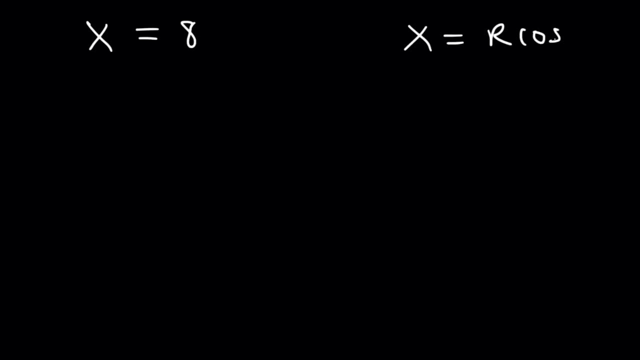 Now we know that x is equal to r cosine theta, so that's the formula we want to use. So let's replace x with r cosine theta, and so that's going to equal 8.. Now, what we're going to do now is we're going to isolate r. 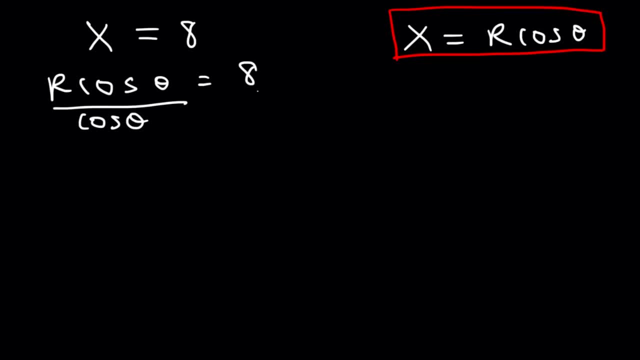 Let's divide cosine, or let's divide both sides by cosine. that's what I meant to say, And so r is equal to 8 times 1 divided by cosine. Now you need to know that secant theta is equal to 1 over cosine. 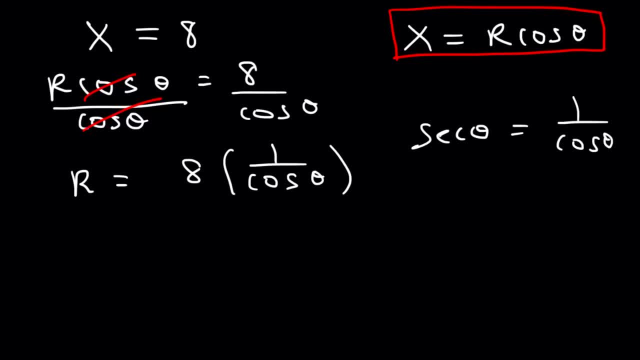 By the way, you could leave your answer like this: 8 over cosine. it should be fine. Or you can write it as 8 secant theta. Personally, I prefer to write it like this, But you could write it as 8 over cosine if you want to. 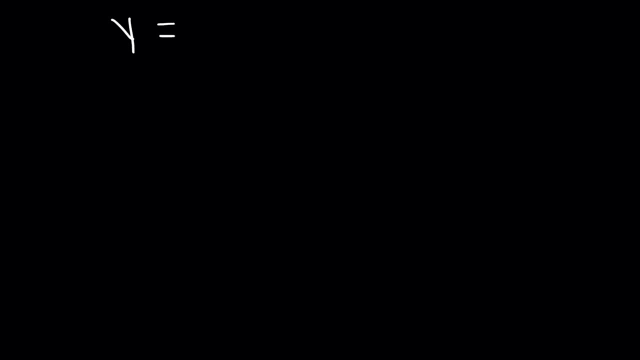 Let's try another similar example. Let's say y is equal to 5.. What's the polar form of this equation? Now we know that y is r sine theta. So therefore, r sine theta is equal to 5.. And now let's divide both sides by sine theta. 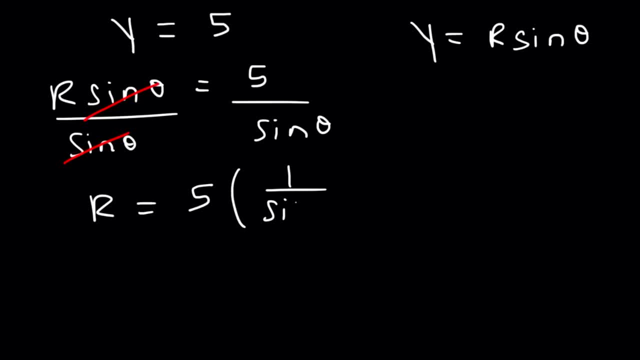 So r is 5.. 5 times 1 over sine theta And 1 over sine is cosecant. So this is 5 cosecant theta, And so that's the answer. Here's another example. Let's say that 5x plus 4y is equal to 8.. 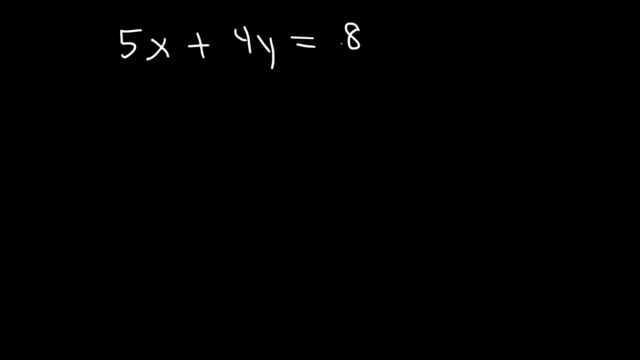 Go ahead and convert that into its polar form. So, as we mentioned before, x is r cosine theta And y is r cosine theta And y is r sine theta. So our goal is to isolate r. If we factor out r- this is a GCF- we'll be left with 5 cosine theta plus 4 sine theta. 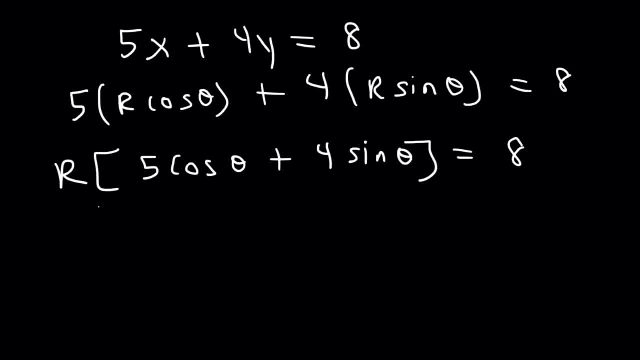 And that's going to equal 8.. So now what we need to do is divide both sides by 5 cosine plus 4 sine, And that's going to equal 8.. So now what we need to do is divide both sides by 5 cosine plus 4 sine. 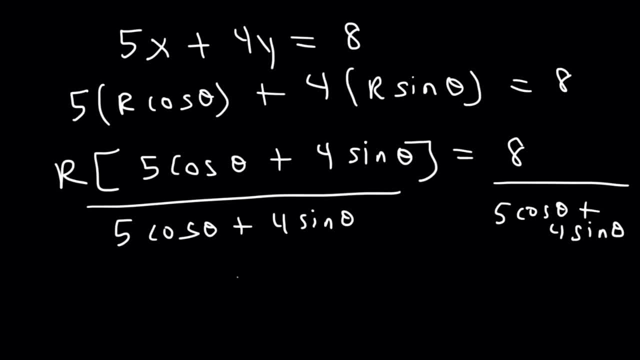 And so now this will give us our final answer. So r is 5 divided by- I mean not 5,, but rather 8, divided by 5 cosine theta plus 4 sine theta. So that's all we can do for this particular example. 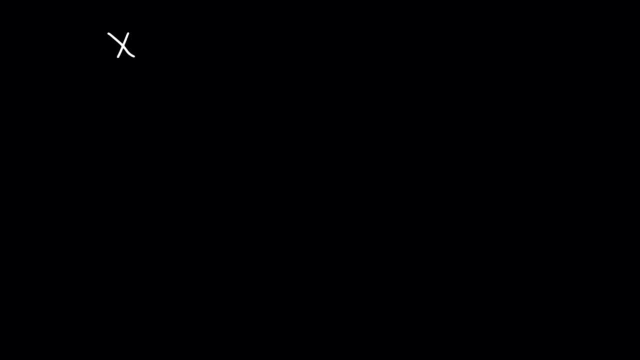 Now, what about this one? Let's say that x squared plus y squared is equal to 8. And x squared is 16. What do we need to do first in this example? So, if we recall, r squared is x squared plus y squared. 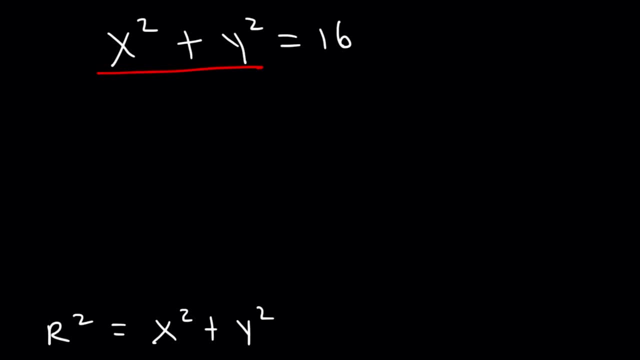 So, therefore, let's replace this with r squared, So r squared is equal to 16.. And now all we can do at this point is take the square root of both sides, So r is equal to 4.. So our goal is typically to solve for r. 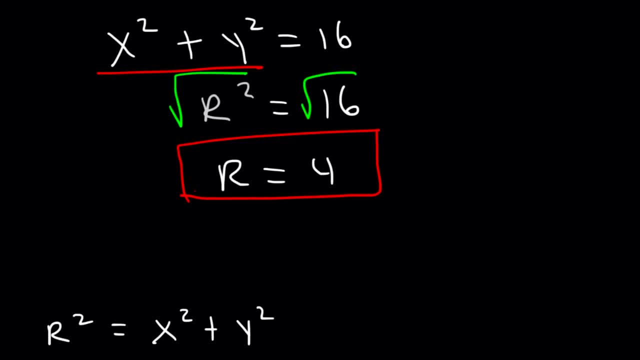 We want to get r by itself on one side. That's usually the case. So that's it for this problem. Here's another one: x minus 3 squared plus y squared, Let's say it's equal to 9.. What's the first thing that we need to do in this example? 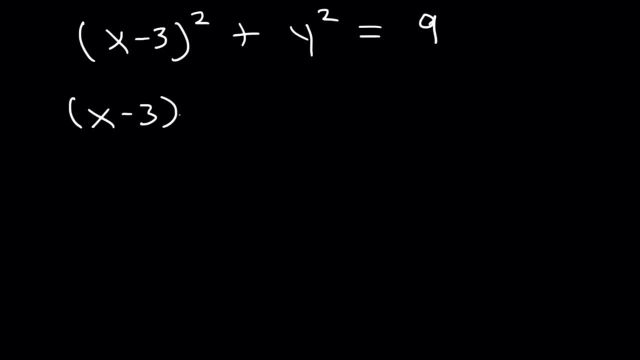 The first thing that we should do is we need to expand x minus 3 squared. It's basically x minus 3 times x minus 3.. Now let's go ahead and FOIL it: x times x is x squared, And x times negative 3, that's negative 3x. 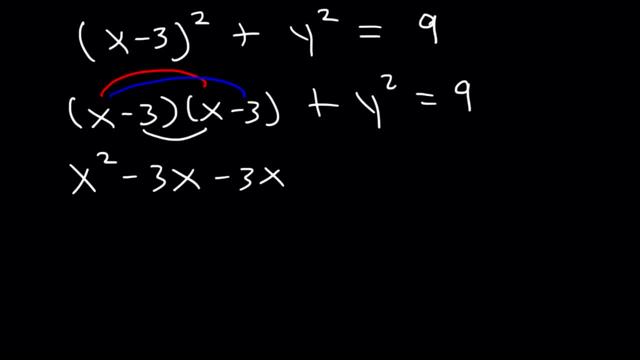 And this is also negative 3x, And then negative 3 times negative 3,, that's positive 9.. So if we subtract both sides by 9, these numbers will cancel And we can also come up with a solution. Combine like terms. 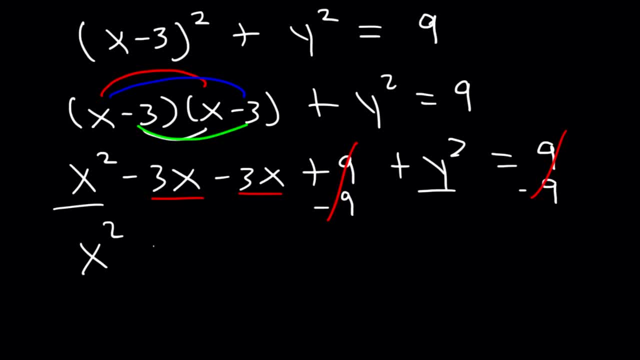 So what we now have is x squared. I'm going to write these two together: x squared plus y squared minus 6x is equal to 0.. Now, if you recall, x squared plus y squared is equal to r squared, So we have r squared minus 6.. 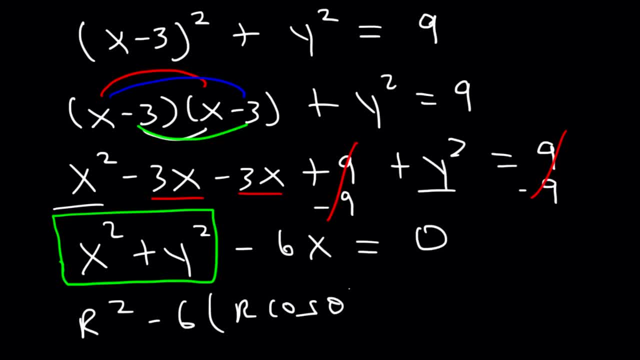 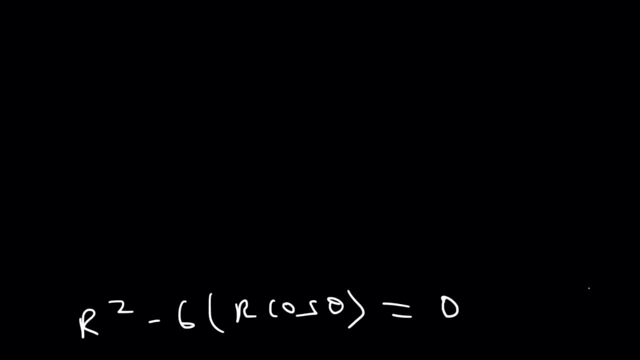 And x is r cosine theta, So that's equal to 0.. So now let's take out an r. If we factor out r, we'll be left with r minus 6 cosine theta, Since r and r minus 6 cosine theta. 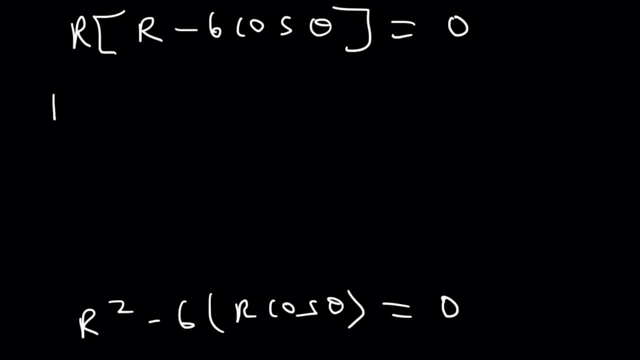 if you multiply them, if they equal to 0, any one of them can be 0.. 0 times anything is 0. So we can set this portion r equal to 0.. And we can set r minus 6 cosine theta equal to 0. 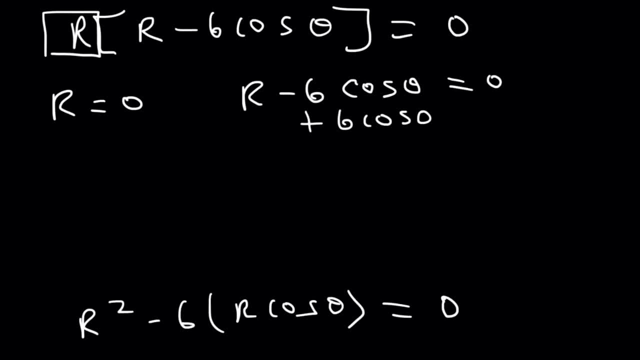 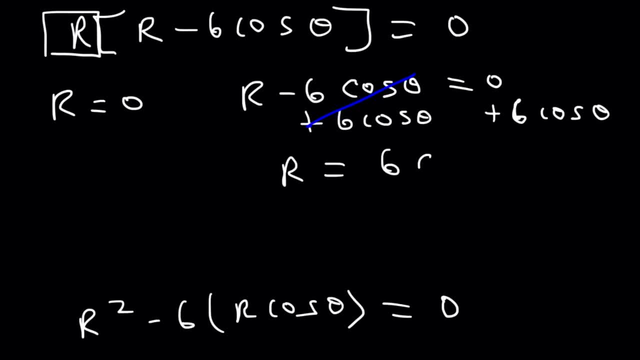 So this gives us two possible answers: r is equal to 6 cosine theta, r is equal to 6 cosine theta, or r is equal to 0.. or r is equal to 0.. Here's another problem. Here's another problem. Let's say that x squared plus. 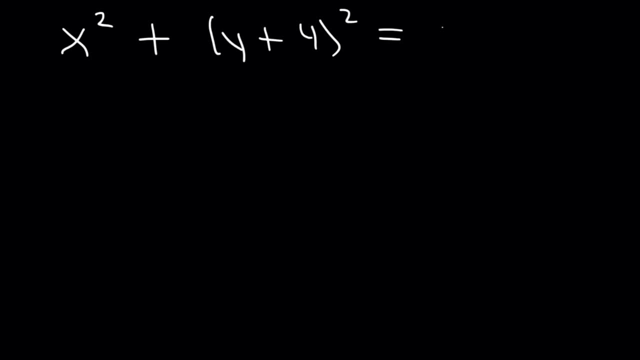 y plus 4 squared is equal to 16.. So, based on the last example, feel free to pause the video and try this one, and try this one. So, just like before, we need to FOIL y plus 4 squared. we need to FOIL y plus 4 squared. 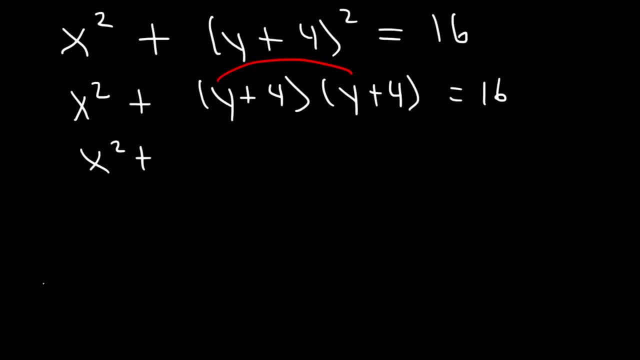 So y times y, that's going to be y squared, And then y times 4 is 4y, And then 4 times y, that's also 4y, And then 4 times 4 is 16.. And then 4 times 4 is 16.. 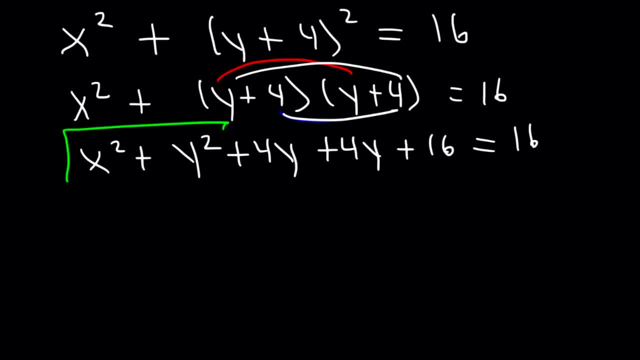 Now we know that x squared plus y squared, we can replace that with r squared. Next, we can add 4y plus 4y, which adds up to 8y, which adds up to 8y, And if we subtract both sides, 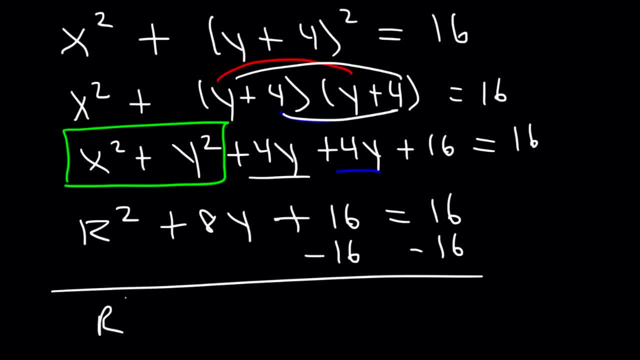 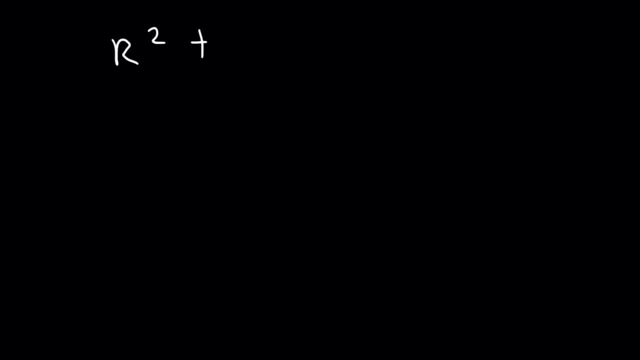 by 16, we're going to have r squared plus 8y is equal to 0.. is equal to 0.. Now let's replace y. Now let's replace y with r sine theta, with r sine theta, with r sine theta. 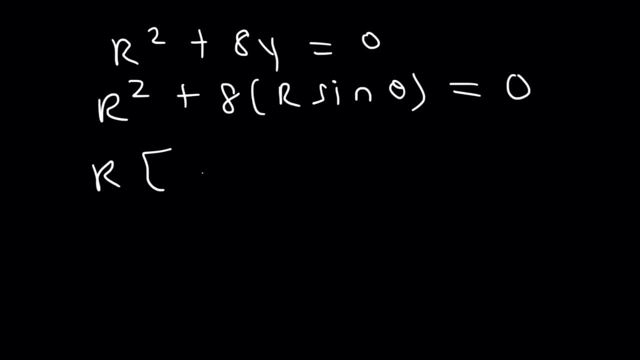 And let's take out an r. So this is going to be r plus 8 sine theta and that's equal to 0.. So now we can set r equal to 0 and r plus 8 sine theta is equal to 0.. 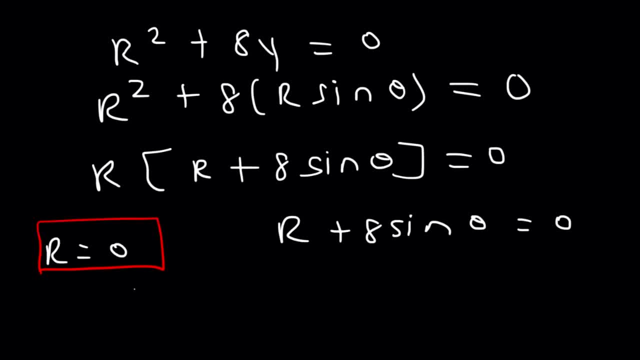 So this is the first answer. and for the second answer, r is equal to negative 8 sine theta. And so that's it. and so that's it. What if y squared is equal to 4x? What can we do to convert this equation? 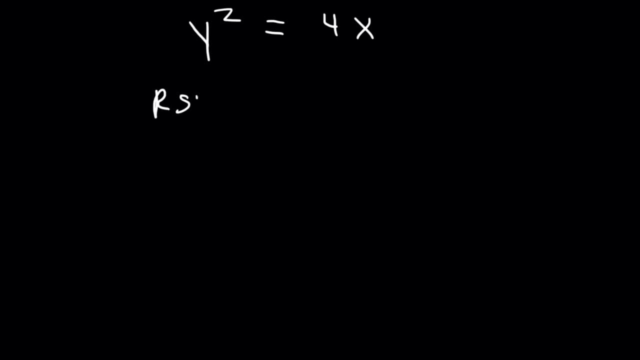 into its polar form. So first we know that y is r sine theta, but since we have y squared, this is going to be r sine theta squared, And x is r cosine theta. So what we have now is r squared sine squared theta is equal to 4r cosine theta. 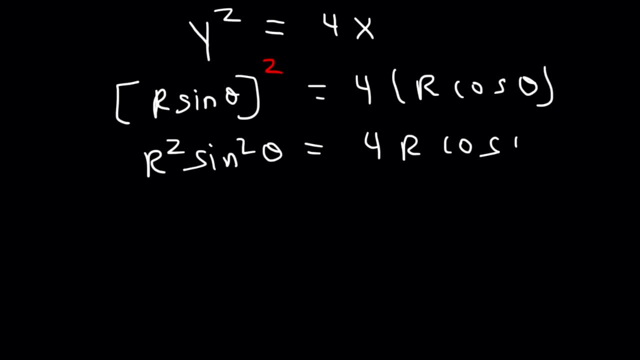 is equal to 4r cosine theta is equal to 4r cosine theta. Now, if we divide both sides by r, at this point we're going to lose an answer, And that answer is: r is equal to 0. Which sometimes some textbooks just completely. 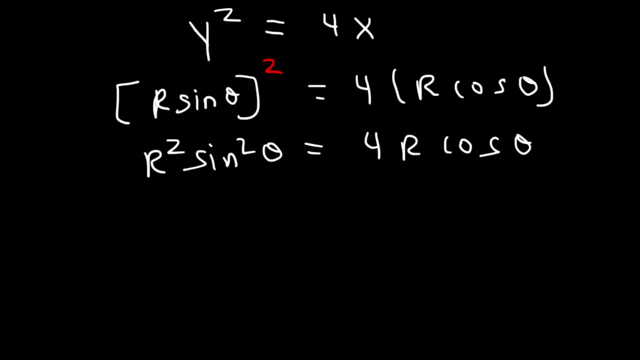 omit that answer, But I'm going to get both answers. So I'm going to subtract both sides by 4r cosine. So basically, I'm going to take this and move it to the left. It's going to be negative on the right side. 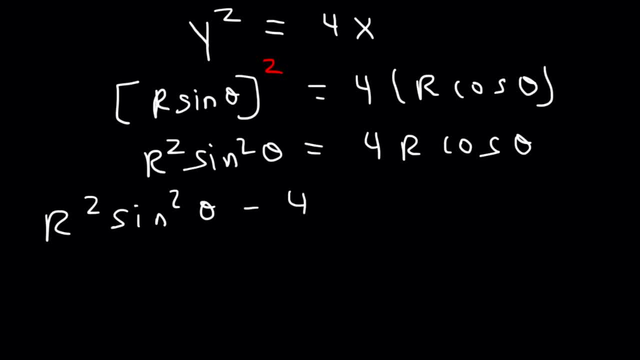 but it's going to be negative on the left side. So I'm going to factor out the GCF, which is r, And I'll be left with r sine squared theta minus 4 cosine theta. So my first answer: r is equal to 0.. 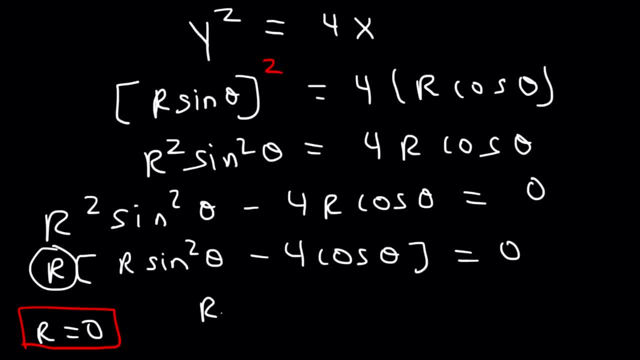 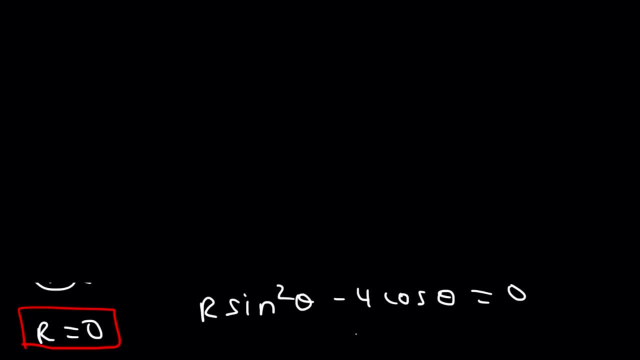 And then the other answer, which is the one that the textbook usually wants: r sine squared theta minus 4 cosine theta is equal to 0.. So we're going to focus on that equation. So I'm going to add 4 to both sides. 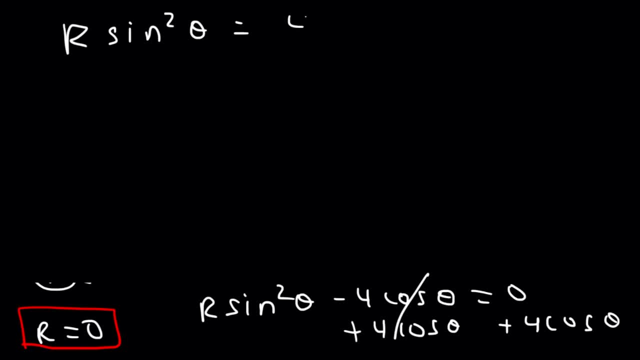 r sine squared theta is now equal to 4 cosine theta, So let's divide both sides by sine squared at this point. So r is 4 cosine theta divided by sine squared, So you can leave your answer like this, if you want to. 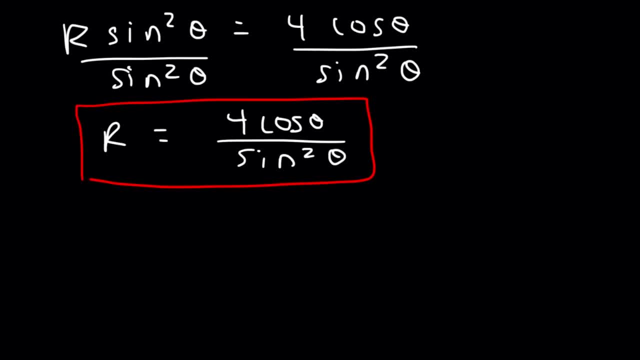 But do know that you can change it also. For example, we can expand sine squared into sine times sine, But I'm going to write it as cosine over sine times 1 over sine. Cosine divided by sine is cotangent And 1 over sine is cosecant. 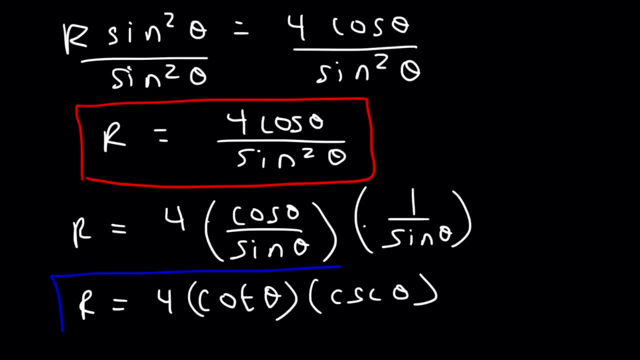 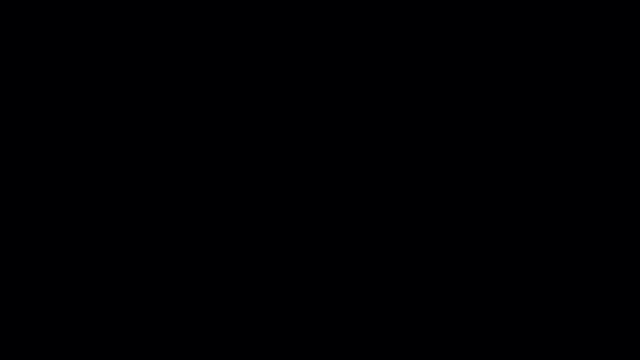 So you could write your answer like this: 4 cotangent cosecant. So both answers are acceptable. Let's work on another similar example. Let's say that x squared is equal to 8y. Try that problem. So we're going to. 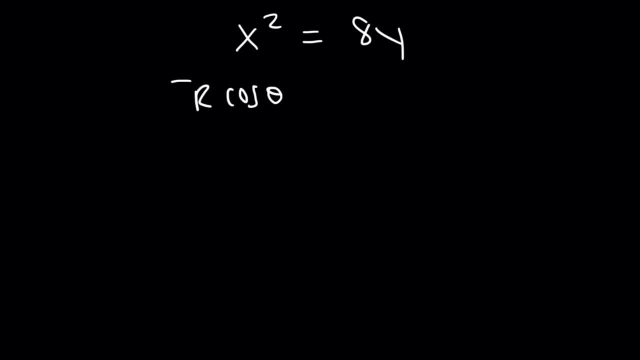 replace x with r cosine theta. Let's not forget to square it. And let's replace y with r sine theta, So r squared cosine squared is equal to 8r sine theta. Now on the last problem. we took the term on the right and moved it to the left. 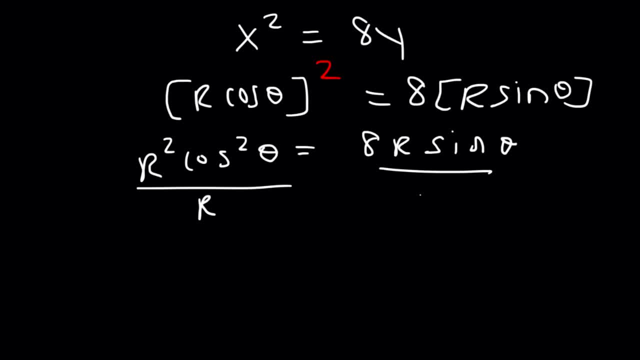 We're not going to do that In this example. we're just going to divide both sides by r. Just keep in mind: when you do this, you lose an answer, And that answer you lose is: r equals 0. Which most textbooks are going to. 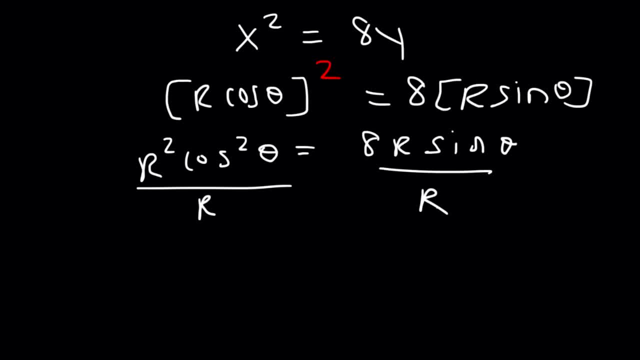 ignore that answer anyway, But just want you to keep that in mind. So we're going to have one r left over on the left side, So r cosine squared is equal to 8 sine theta. And now let's divide both sides by cosine squared. 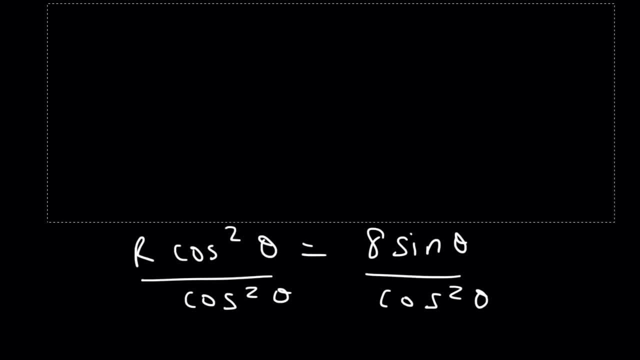 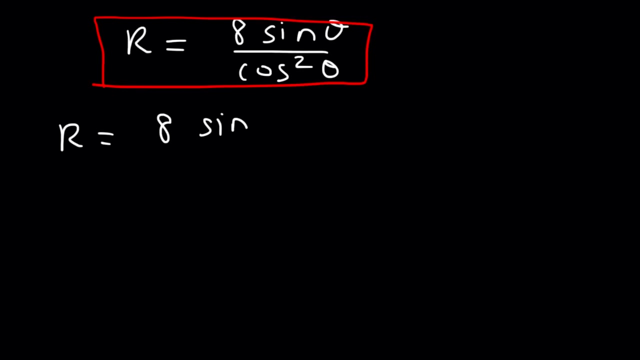 So now we have the answer: r is equal to 8 sine theta divided by cosine squared. But now let's change it. So let's rewrite it as sine divided by cosine times 1 over cosine. Now, sine over cosine is equal to: 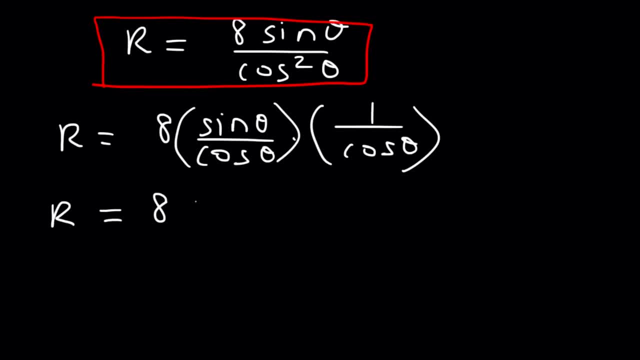 what other trig function? Sine divided by cosine is tangent theta And 1 over cosine is secant theta. So therefore r is 8 tangent theta, secant theta. Now what about this problem? x squared plus y squared, Let's say: 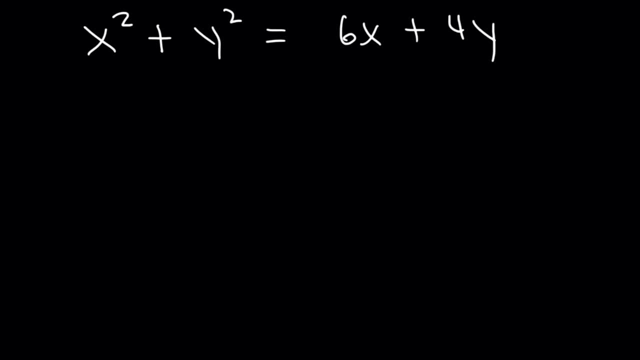 it's equal to 6x plus 4y. Try that. So we know that x squared plus y squared, that's equal to r squared, And x is r cosine theta y. we know it's r sine theta. 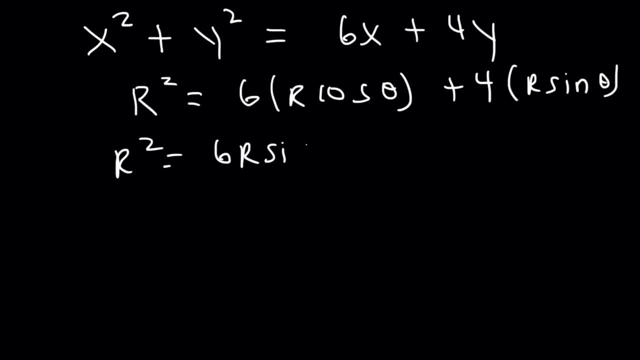 So r squared is equal to 6r sine theta. I mean not sine, but cosine theta. Now, what do you think we should do at this point? At this point, what we need to do is divide each term by r. 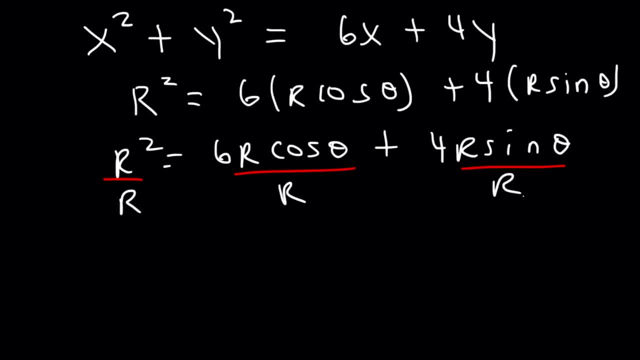 And keep in mind, we'll lose the answer. r equals 0.. So you can just add it towards the end. So right now we have: r is equal to 6 cosine theta plus 4 sine theta. So that's the equation that we want. 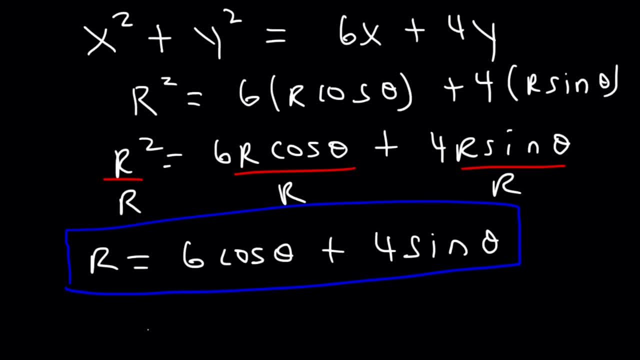 But keep in mind that r can be 0. Because 0 squared and 6: 0 squared is equal to 6 times 0 times cosine plus 4 times 0 times sine. Because if this is equal to 0 and that's equal to 0. 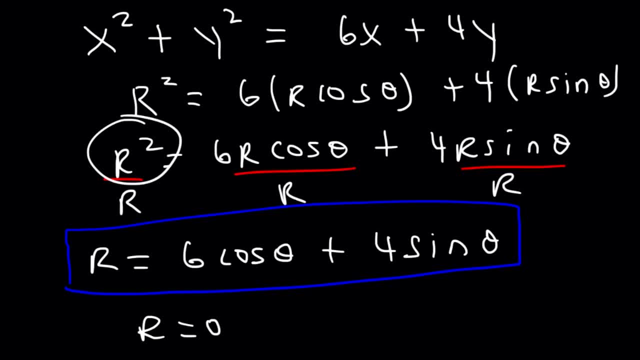 then this will be equal to 0 as well, So 0 will make that equation true, But the answer that we want is this one: r is equal to 6 cosine theta plus 4 sine theta. Now, what about this one? 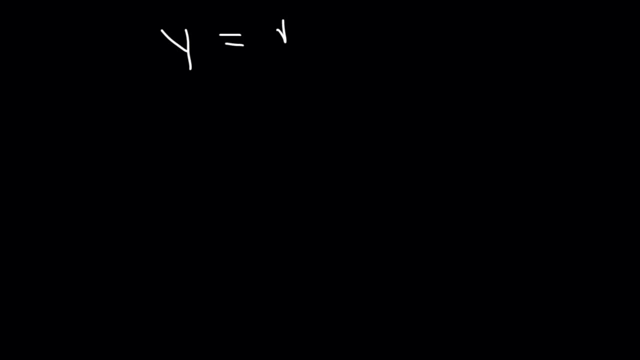 Let's say y is equal to the square root of 3 times x. Let's convert that equation into its polar form. So y is equal to r sine theta and x is r cosine theta. So if we divide both sides by r,